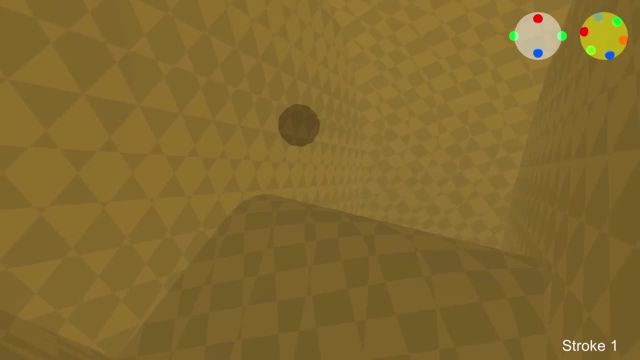 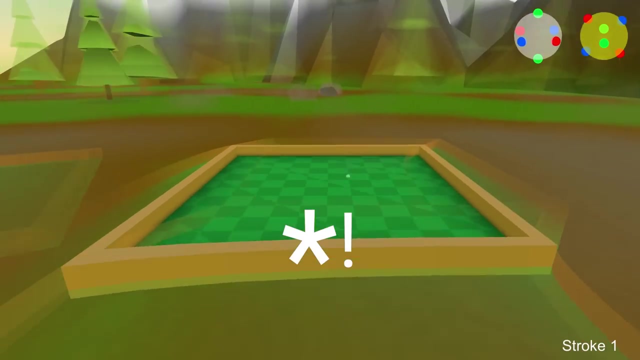 view. Okay, but then there's not really a difference with a regular 3D game. it's just like a different view. But remember that big asterisk- we're assuming no change in height. Some earlier levels are flat, but once you start getting to the slopes and other terrain, 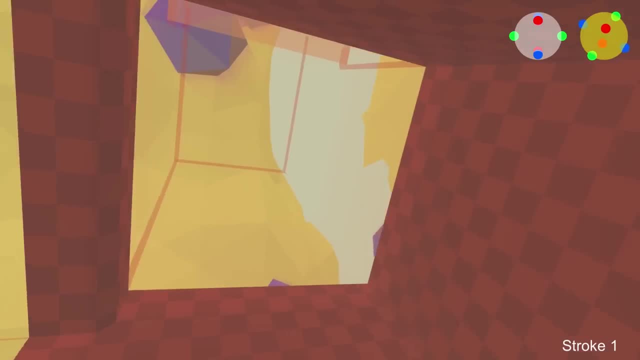 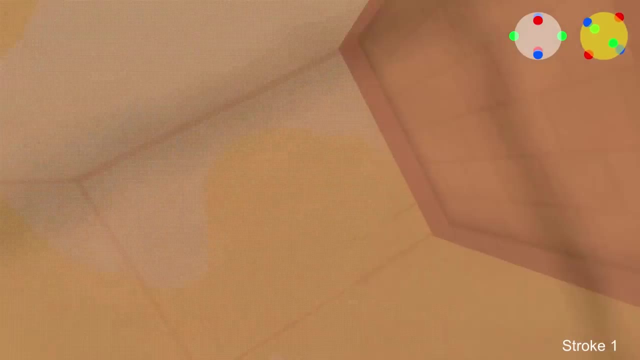 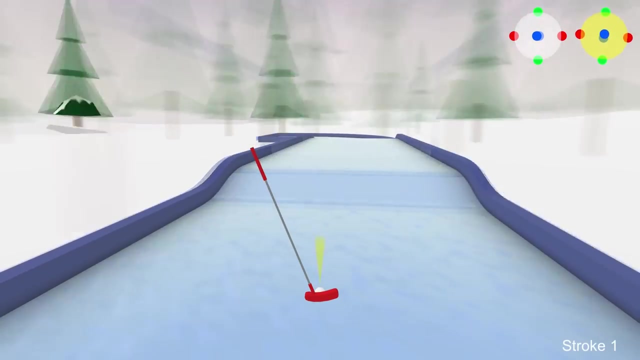 that model breaks down, Which is good. I want that 4D experience. Regardless, it's still a really useful view of the space, especially when designing levels. One of my goals for 4D Golf is that I don't want the navigation and movement to be the challenge. 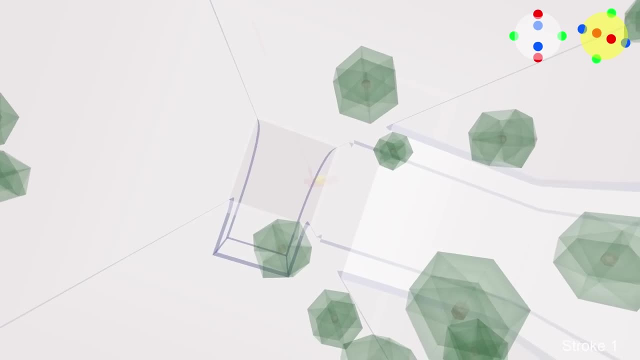 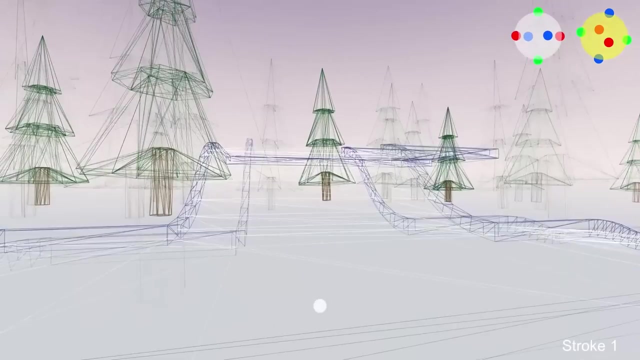 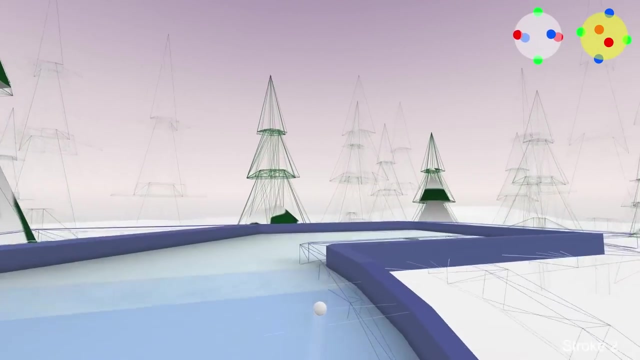 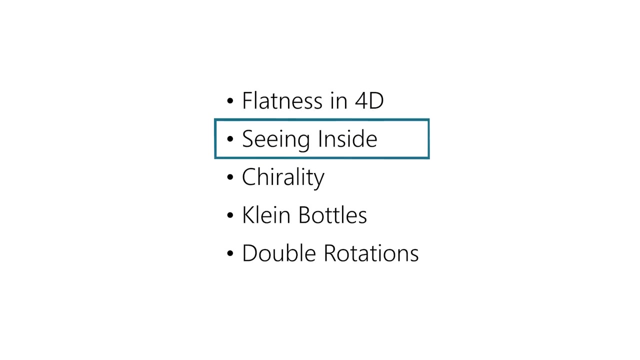 of the game. That should be as easy as possible, which is the reason I have so many different visual and control options. The 4D stuff is there to give new golfing challenges that are fun to play. So do you get Superman's x-ray vision in 4 dimensions? Well, that's a statement I've seen. 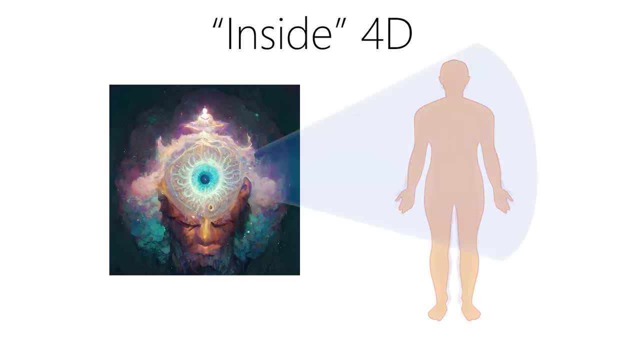 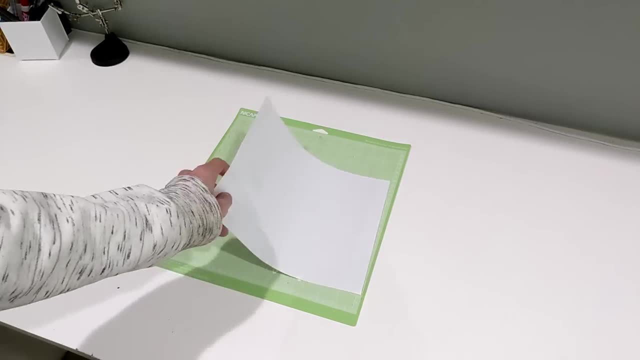 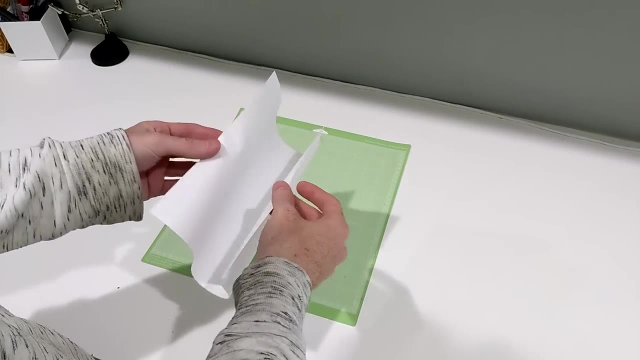 a lot about 4D that you can see inside of 3D objects, like the organs in your body, But semantically that's really misleading. Just like how we can't have infinitely thin paper in our universe. there's no such thing as a physical 3D object. in 4D, Everything needs some kind of. 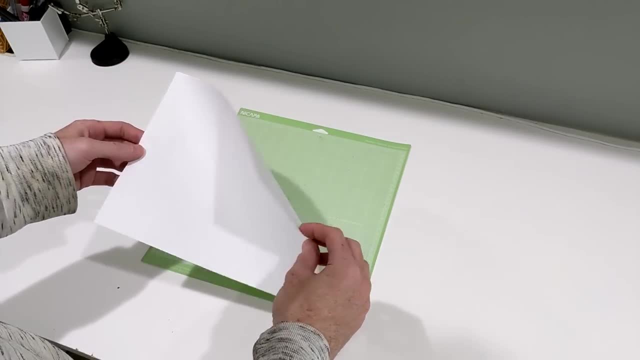 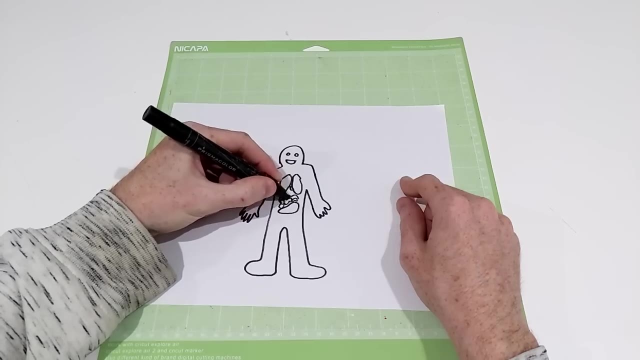 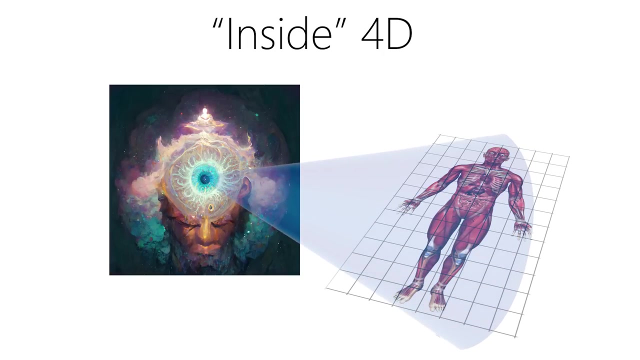 thickness And if you have paper you don't see or draw things quite right inside. We draw on top of the paper. In that way, the word inside means something completely different to a four-dimensional being. 3D things are flat, so they'd see the top of this flat person. That means all 3D things have a. 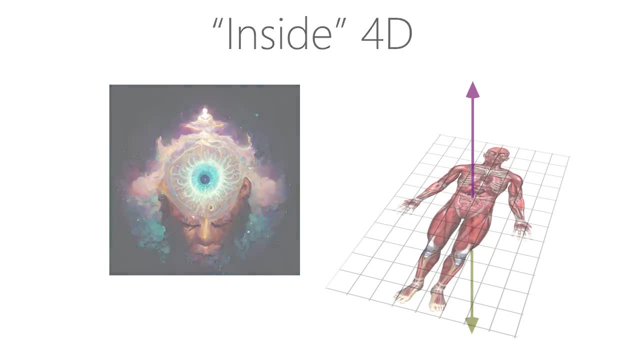 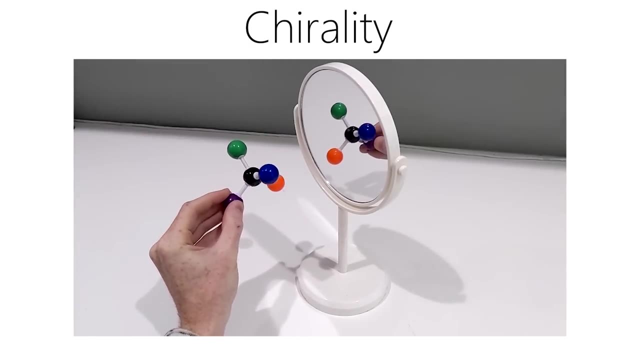 4D top and bottom. And that brings me to my next point. Would you be able to tell your left hand from your right? Chirality, or the ability to tell left from right, doesn't exist for 3D objects anymore, even if they have a thickness Like 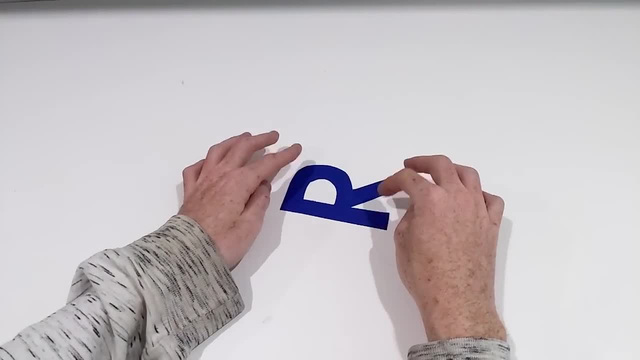 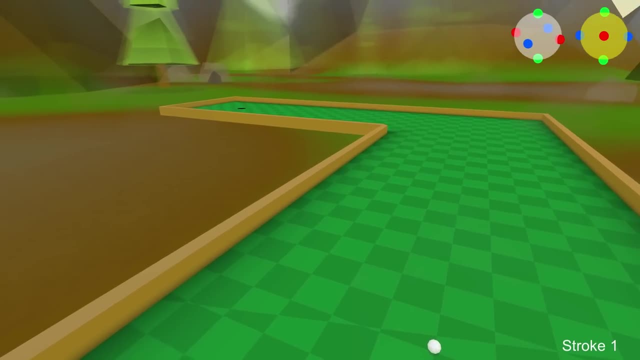 normally, if you have a paper cutout, you can't make a mirror image by just rotating the paper in its plane. You'd have to turn it over. in the third dimension It's the same for flat objects in 4D. Here it looks like the hole is on. 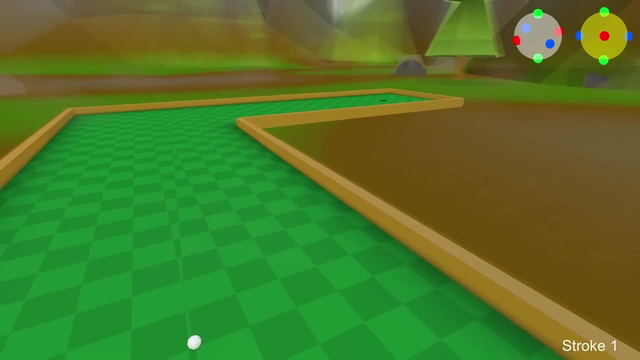 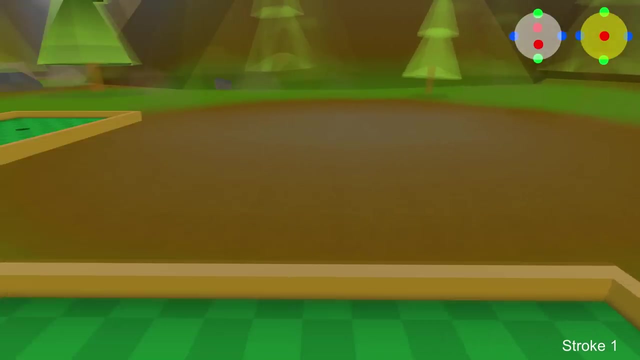 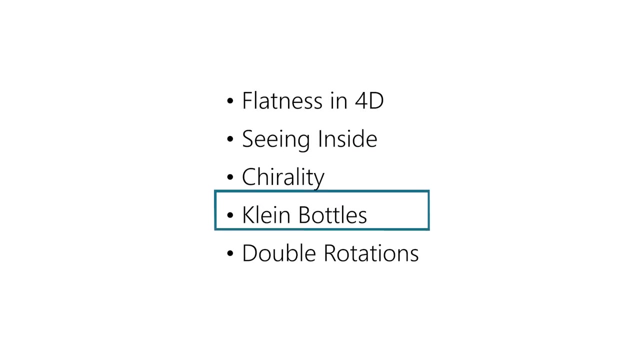 the left, but maybe it's actually on the right side. Unlike the paper, you can rotate your view to see a mirror image. Pretty cool. For something to be identified as left or right-handed now it needs differences in all four dimensions. I can't pass up an opportunity to talk. about a 3D object in 4D. I can't pass up an opportunity to talk about a 3D object in 4D. I can't pass up an opportunity to talk about a 3D object in 4D. I can't pass up an opportunity to talk. 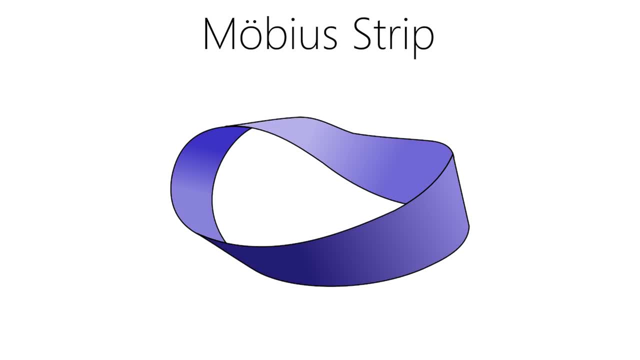 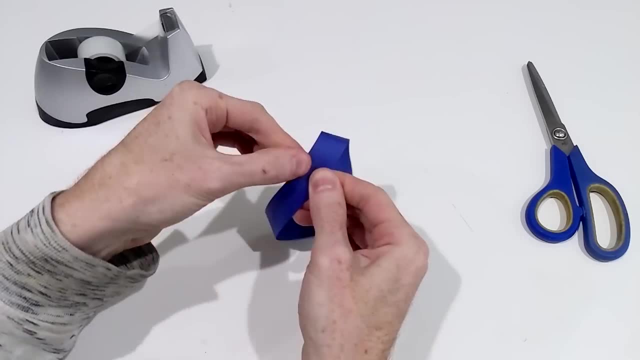 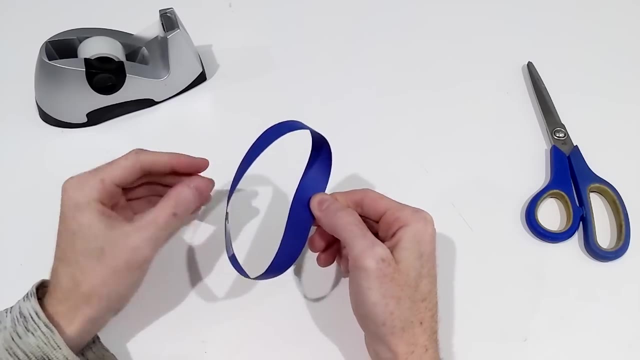 about Klein bottles. Are you familiar with the Mobius strip? You start by cutting out a rectangular piece of paper, add a twist and then tape the ends together. The total area of the paper didn't change, but it went from having two sides to one side and a boundary of two edges to one edge, If you were to. 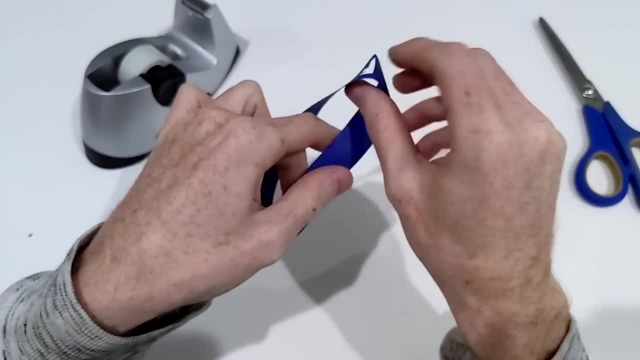 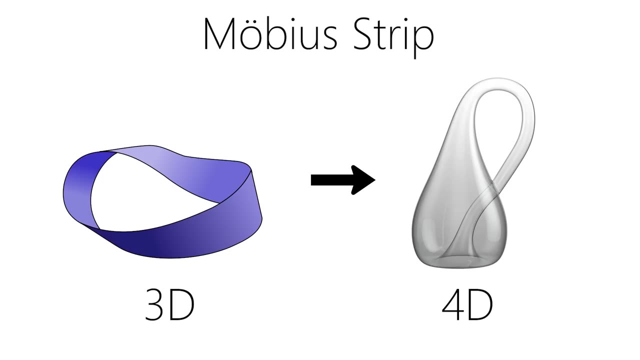 send a right hand down the strip, it would come back to the other side as a left hand, if you could see through it. So how do we bring the Mobius strip a dimension higher? It's a Klein bottle, right? Actually, no, the Klein bottle is just another two. 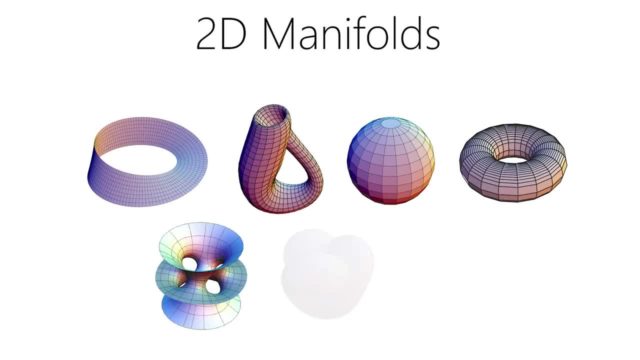 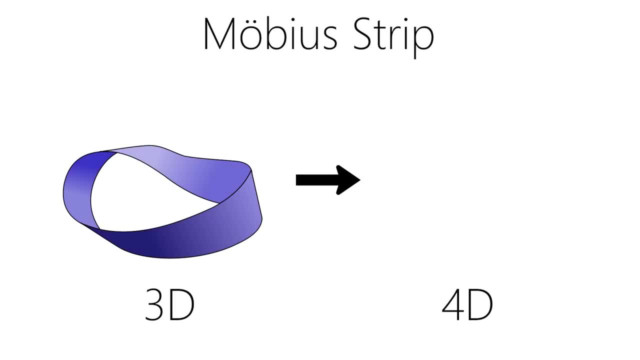 dimensional manifold like any of these other surfaces. In fact, no matter how complicated they are, all 2D surfaces can be embedded in 4D without intersection. No, what we have is something called a solid Klein bottle. This is not an object. 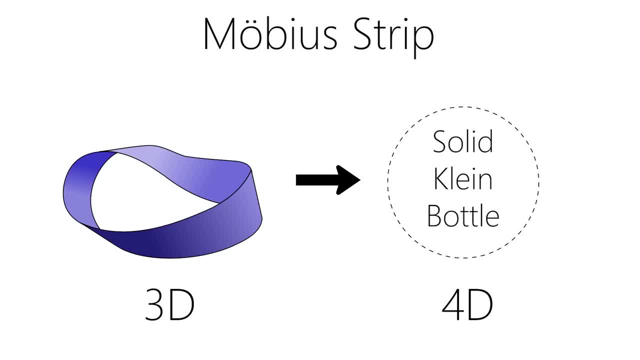 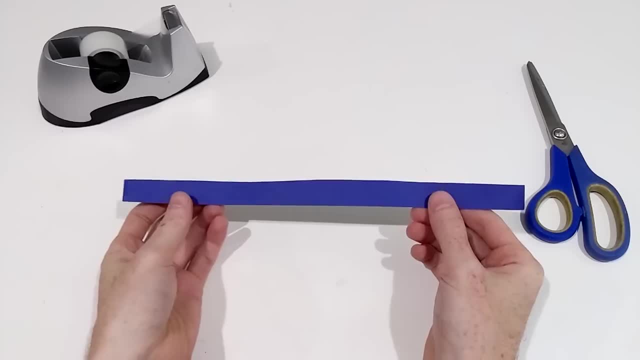 that exists in 3D, but let's try to understand it using everything I've talked about so far. First, let's replay that again and I'll describe it in a 4D context. this time We start with a flat cylinder. Remember 3D, things are flat. 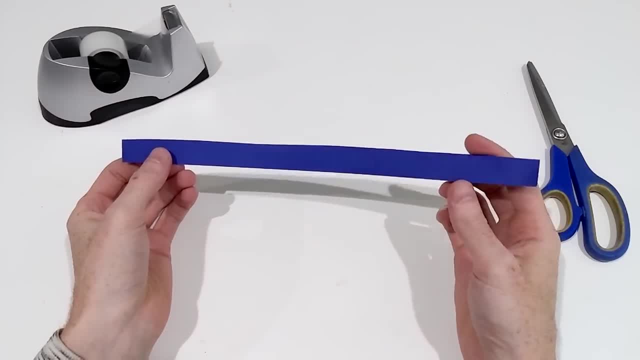 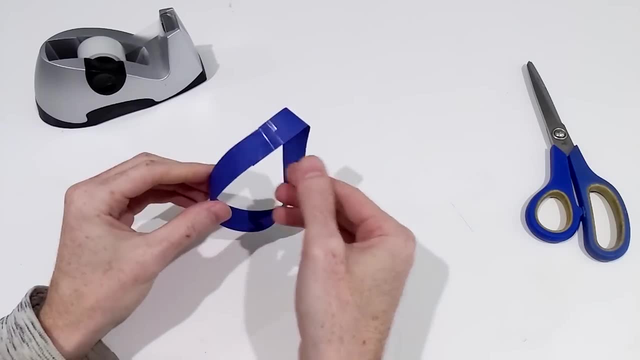 and they have a 4D top and bottom. Then we give it a twist in the fourth dimension and tape the surfaces together. The volume didn't change, but now it only has one side in 4D. If you send a 3D right, hand down the strip, it'll come. 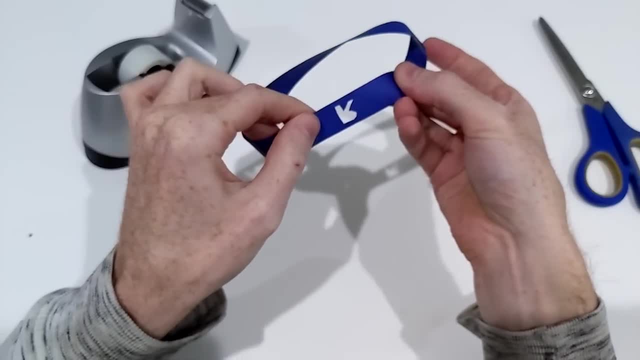 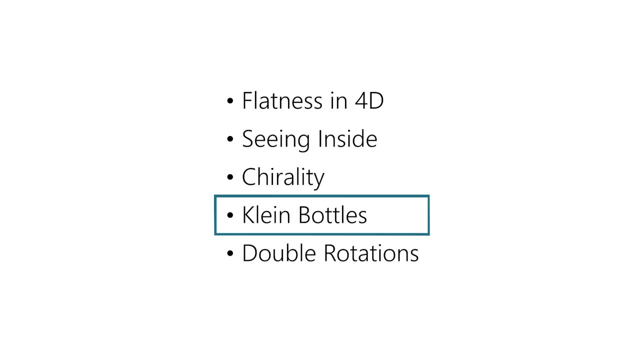 back as a left hand, And the boundary of the solid Klein bottle is the familiar 2D one. Now you're thinking in four dimensions With me, so far Kind of Well. this is the part where it's gonna get a little trickier. 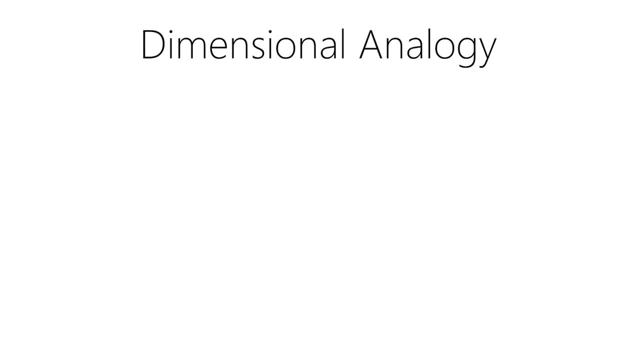 So far, everything I've talked about has had dimensional analogies, where you can think about something in two or three dimensions and kind of naturally extend it to 4D. But some things are entirely new and double rotations are the best example. So in 2D and 3D we usually think of rotations as rotating.